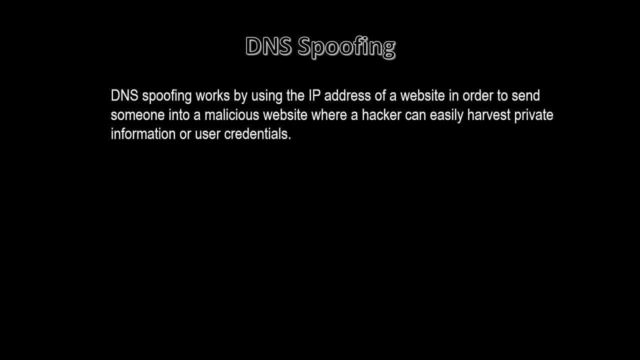 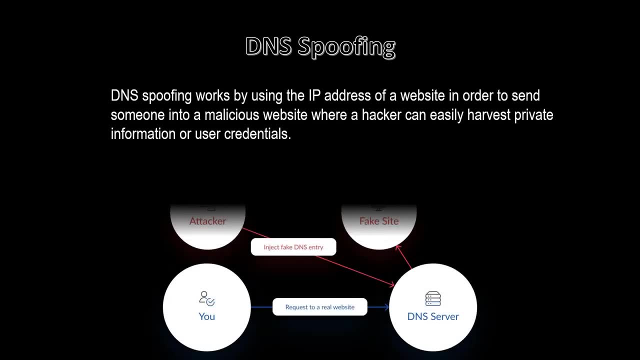 malicious website where a hacker can easily harvest private information or user credentials. this man in the middle attack allows you to communicate with an unsuspecting target into thinking that he has entered a website that he searched for, and then allow a hacker to freely receive account details that this user will be entering on a false website in order for this. 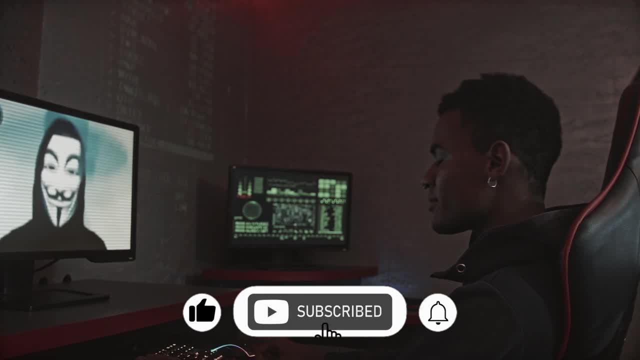 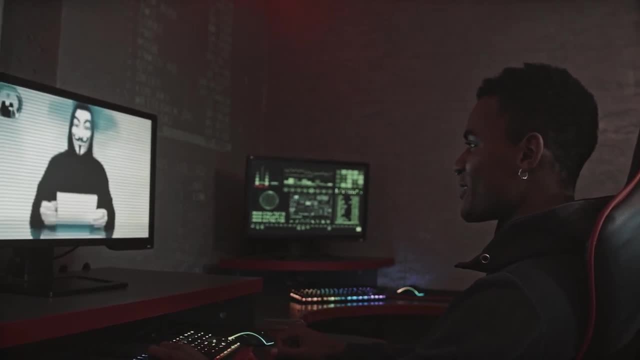 to work, the hacker needs to be on the same land as the target. in order to acquire active UhU 뜻 thai, A hacker can simply search for a weak password on a machine that is connected to that network, which can even be done remotely. 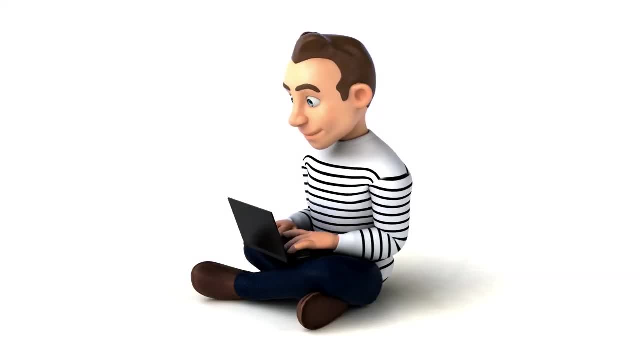 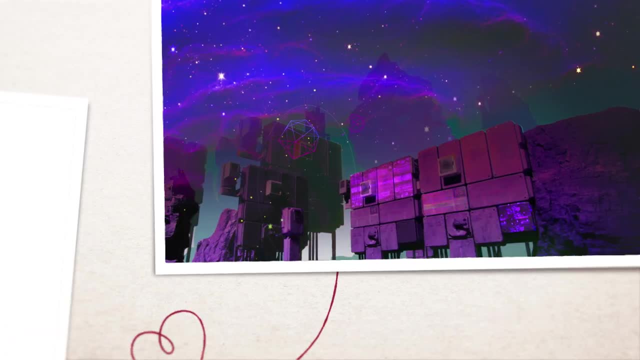 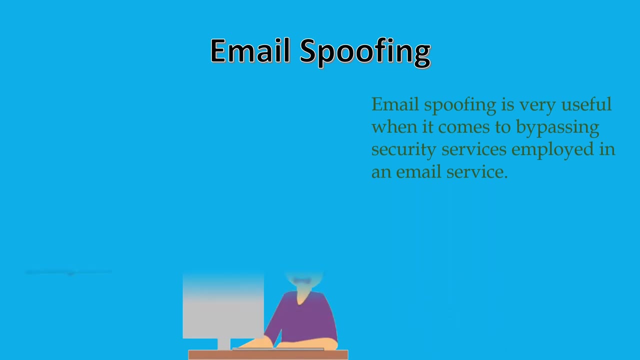 Once this is done successfully, a hacker can redirect users to go to a rigged website and monitor all activities that they will do there. The third is email spoofing. Email spoofing is very useful when it comes to bypassing security services employed in an email service. 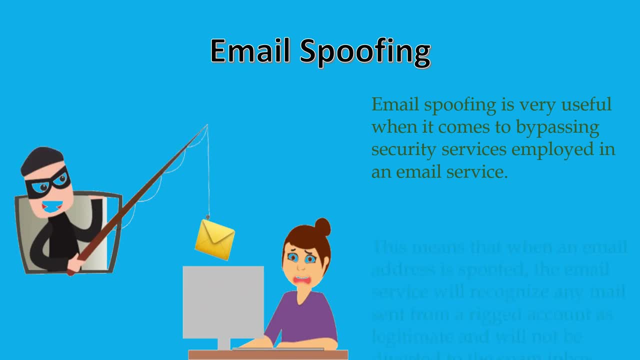 This means that when an email address is spoofed, the email service will recognize any mail sent from a rigged account as legitimate and will not be diverted to the spam inbox. This technique allows a hacker to send emails with malicious attachments to a particular target. 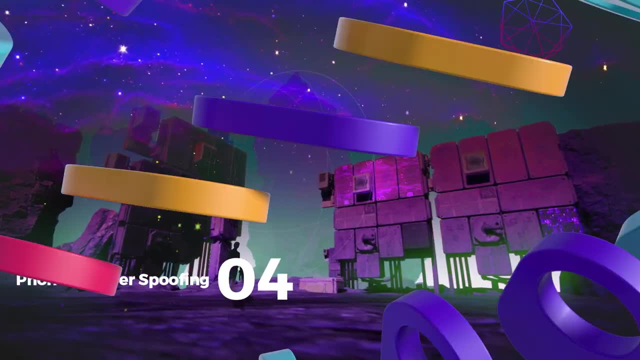 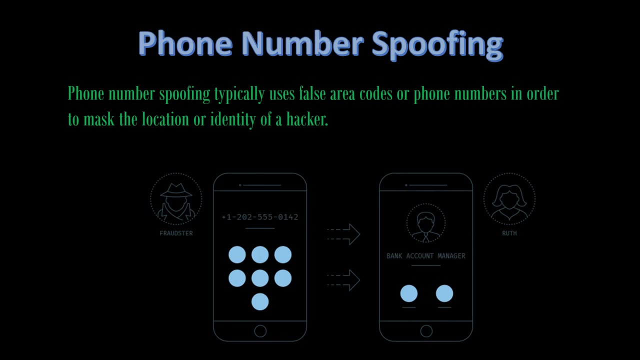 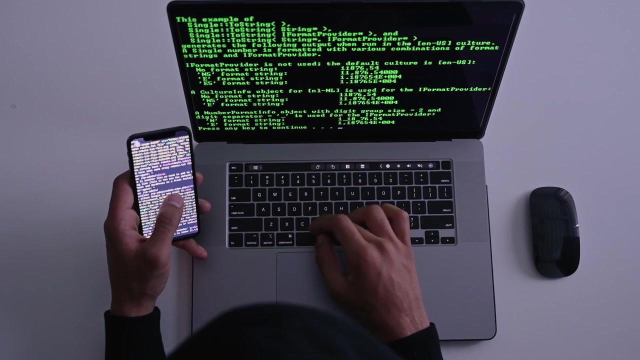 The fourth is phone number spoofing. Phone number spoofing typically uses false area codes or phone numbers in order to mask the location or identity of a hacker. This tactic allows hackers to successfully take a spoof. For example, hackers can tap voicemail messages of their targets, send text messages using a spoofed number or mislead a target from where a call is coming from. 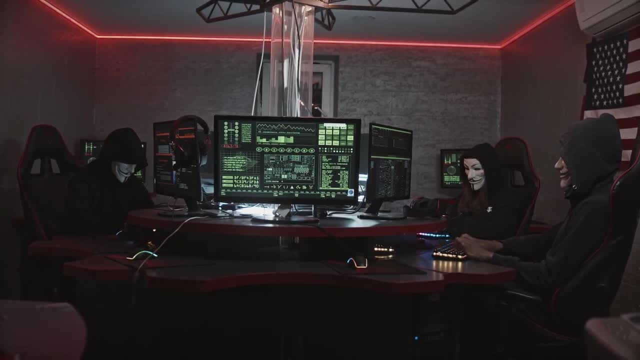 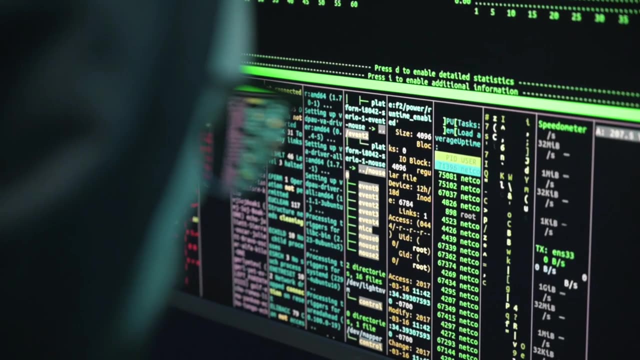 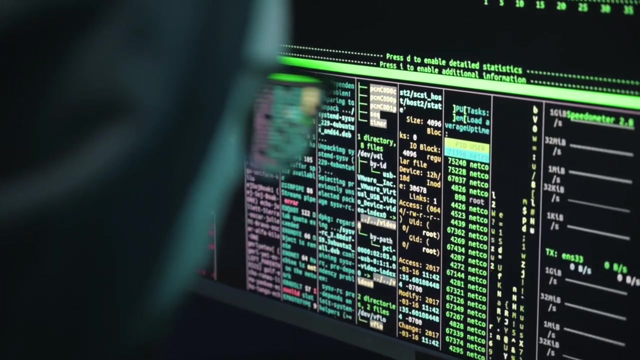 All these tactics are very effective when laying the groundwork for social engineering attacks. The damage of masquerading or spoofing attacks lies on the fact that they are not easily spotted by most network administrators. The worst part is that network administrators and the installed security protocols allow malicious users to interact with other users over the phone. 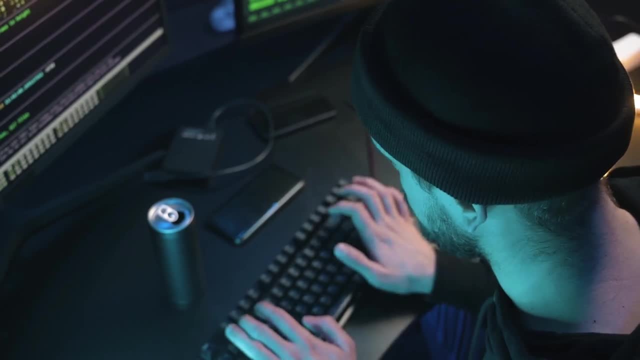 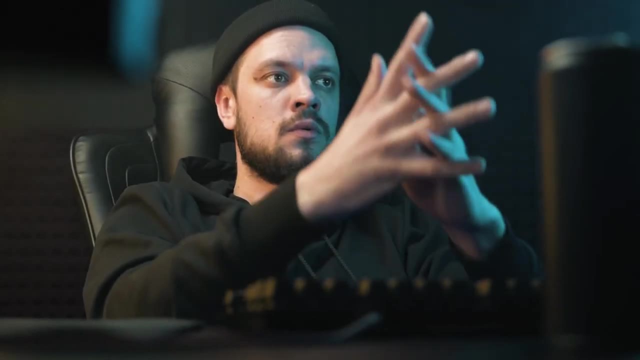 A hacker can even manipulate, stop or inject data stream into the targeted system. Because a hacker that is able to infiltrate the network can easily set up shop in one of the hosts or manipulated devices in the system, it becomes easy for him to conduct man-in-the-middle attacks.